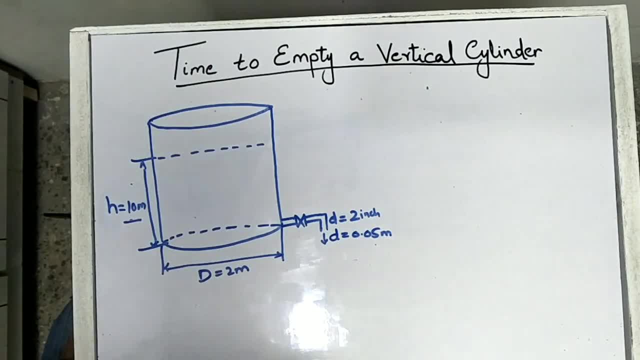 inches. converting into meter is 0.05 meter. So its formula is very simple: Pi constant d square divided by CD, constant area of orifice means area of this drain point multiplied by height of water fill level. d divided by 8 into g, where g is acceleration due to gravity or gravitational acceleration. 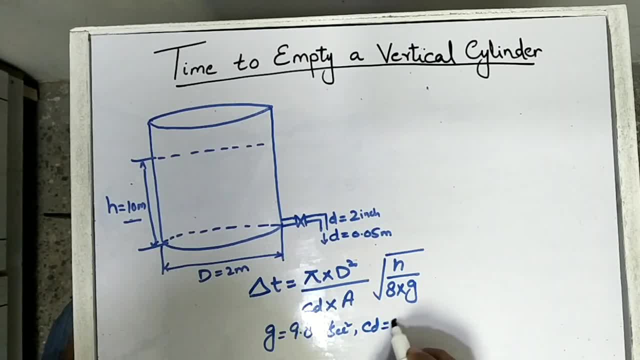 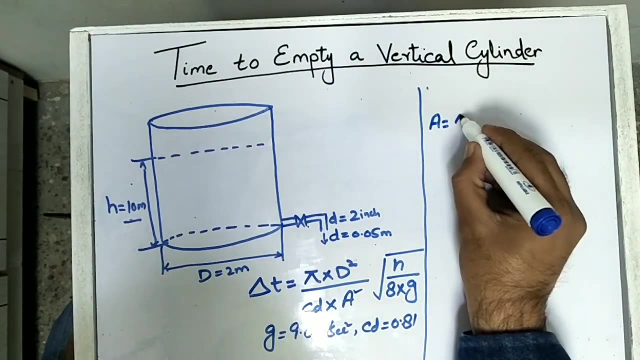 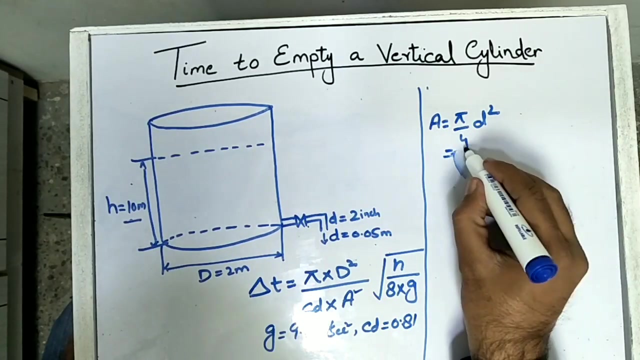 where CD is constant and its value is 0.8, when Now, first of all, we need to calculate this area of this orifice, and, as we already know, the formula of area is pi by 4. square, so, value of pi is three point one, four, four, and area and diameter of 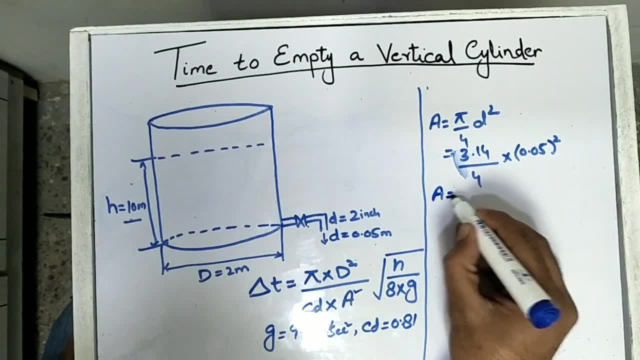 orifice is point zero five. so we get area, point double zero, two meter square. so now all values. we know pi, we know diameter, two meter height, we know ten meter area. we have calculated: and G is nine point eight meter per second square and CD is point eight one. now putting all values three point one, four into two. 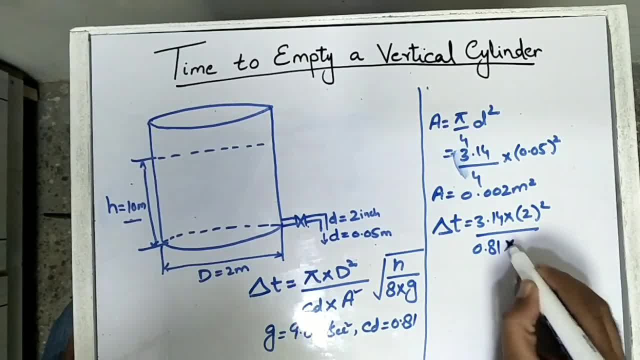 meter square, point eight, one point double zero, two. and height is ten meter, divided by eight, into nine, point eight. now, solving this part, first of all, we will get double seven, five, three. now, solving this part, we will get point three, four, six, four. multiplying these two, we will.